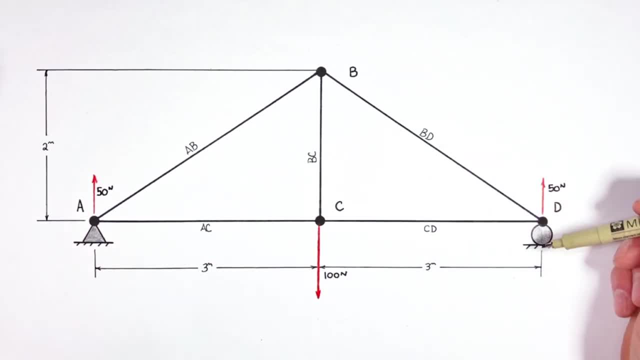 center, then finding the reaction forces would be a bit more complicated, but let's save that for another day. With this first truss, we're just trying to keep things as simple as possible. Now. the next step in analyzing this truss is solving for the forces in each of these beams. 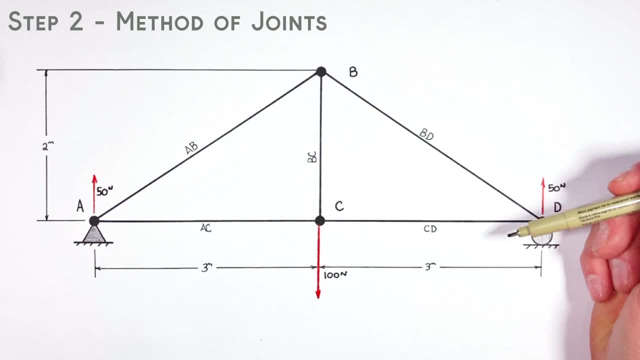 And to do that we're going to use something called the method of joints. You see, the method of joints takes a look at all the forces acting on each individual joint, And those forces can be produced either by the beams that make up the truss, the supports that are holding up the truss, 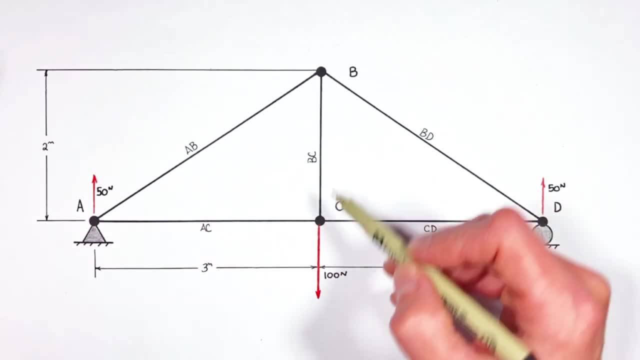 or the load itself. Now we're going to apply the method of joints to each of the joints in this truss, And the question always comes up: well, which joint should we begin? Well, the fact of the matter is, you can typically start either at either of the supports. 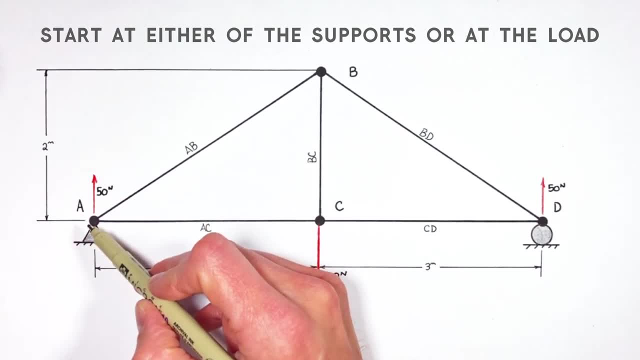 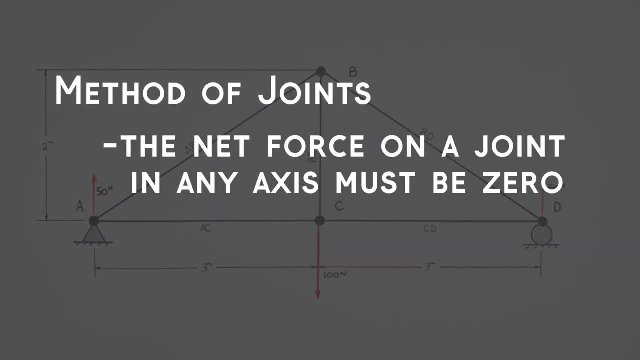 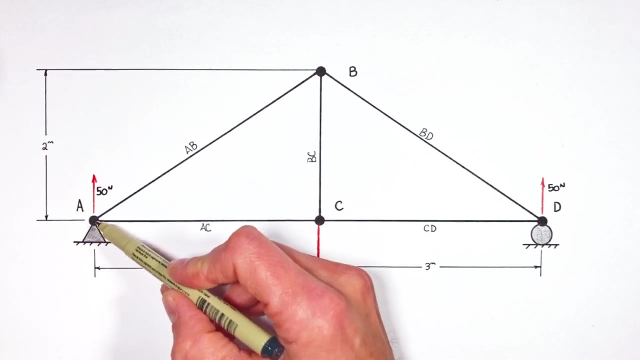 or the load. So today let's start over here at joint A. You see, the method of joints boils down to one simple idea, and that is that the net force on a joint in any axis must add up to zero. That is to say, all the forces acting on this joint vertically must add up to zero. 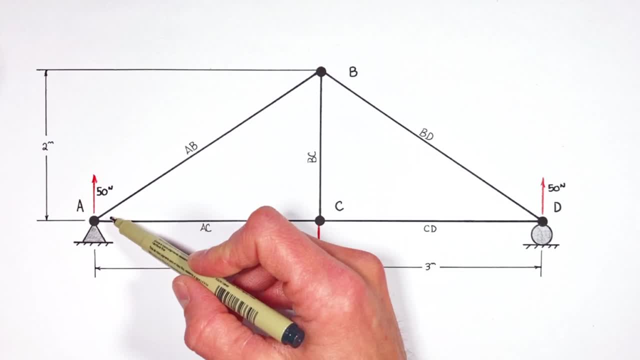 and all the forces acting on this joint horizontally must add up to zero. Now there's three things which are acting on this joint. right here There's these two beams, as well as the support, And you already know the support is pushing up with a force of 50 newtons, which means 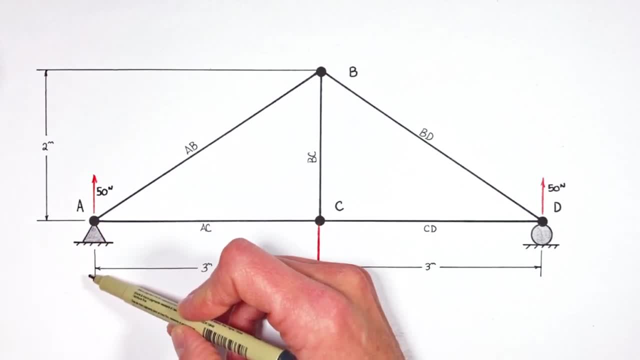 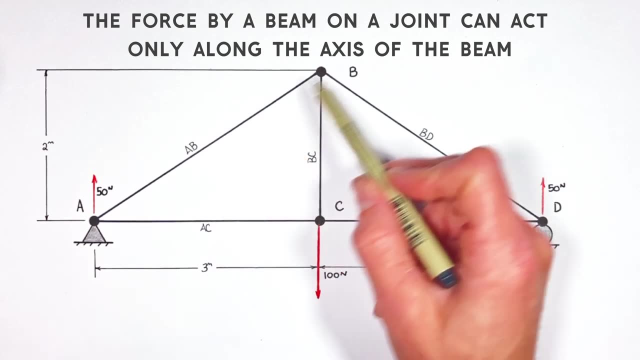 something must be pushing down on this joint with a force of 50 newtons. Now there's a rule anytime you're solving trusses, and that is that any individual beam can either push on a joint or pull on a joint, but it can't produce any torque. That is to say, this beam right here. 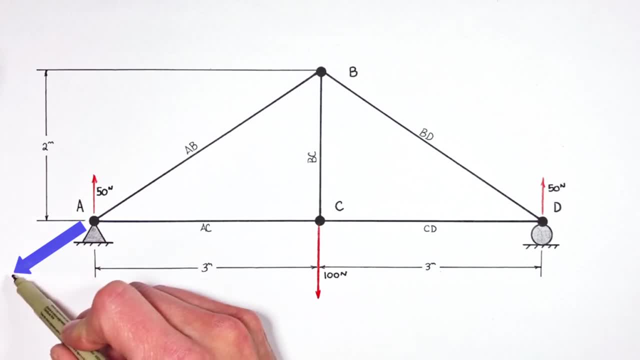 beam AB can either push down to the left on this joint or pull up and to the right on this joint, but it can't act straight. So you can see that the support is pushing up with a force of 50 newtons. 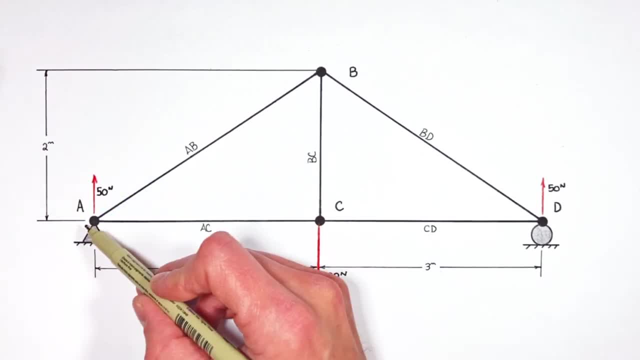 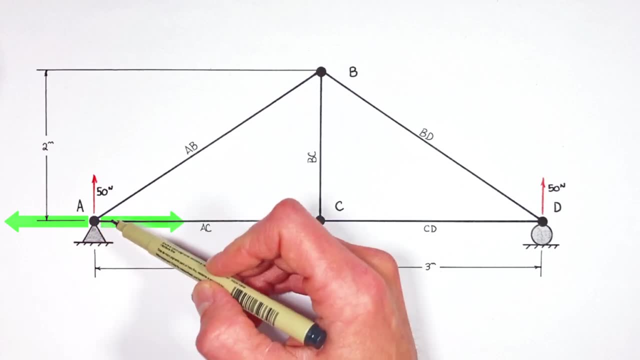 down on the joint. In a similar manner, AC can either act horizontally to the right or horizontally to the left on this joint, but it can't act vertically. So going back to the idea that the total force on this joint in the y-axis must add up to zero, that means something. 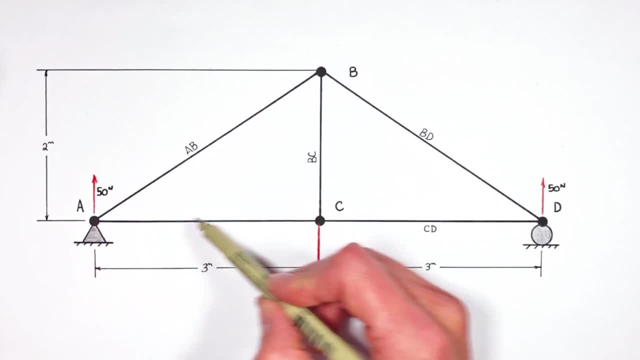 has to be pushing down on this joint. Since AC is a horizontal beam, it can't be beam AC pushing down. That means AB must be pushing down with a force of 50 newtons And the only way for beam AB pushing downward is for the beam to actually be producing a force down and to the left And really 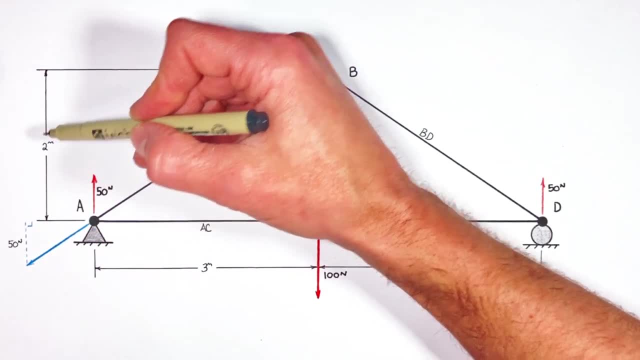 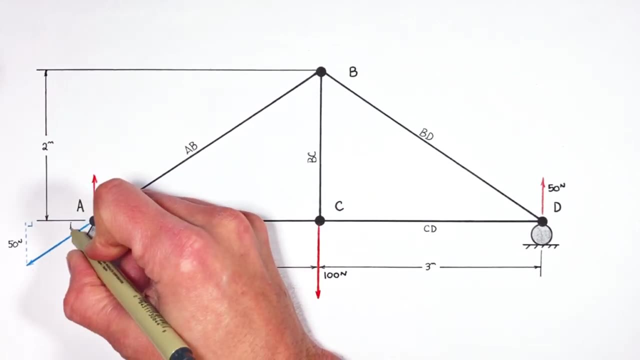 all we have now is a right triangle. Now, given the dimensions of this truss, we know this angle right here is 33.7 degrees, which means this angle right here is also 33.7 degrees. So, going back to right triangle trig, knowing the opposite side of this triangle as well as the angle, we can solve for 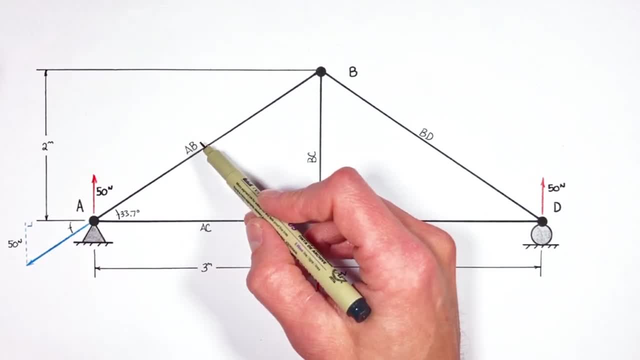 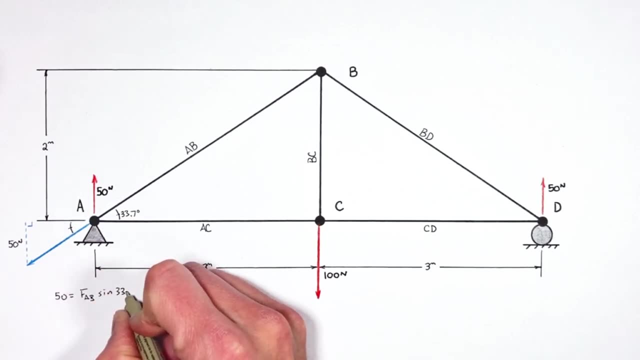 the hypotenuse, that is, the force produced by beam, AB. So, setting 50 equal to the force in AB, multiplied by the sine of 33.7,, we find the force in AB is 90.1 newtons. And knowing the force in AB, we can now solve for the force in AC. You see, since AB is, 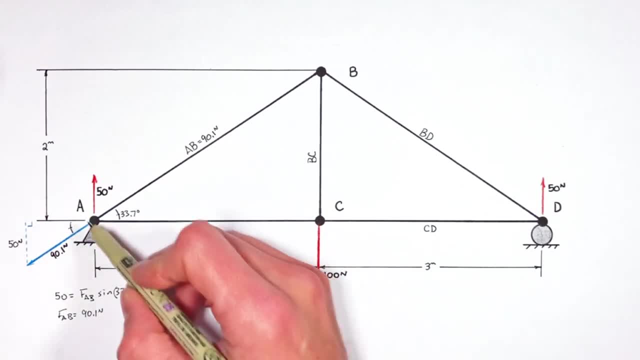 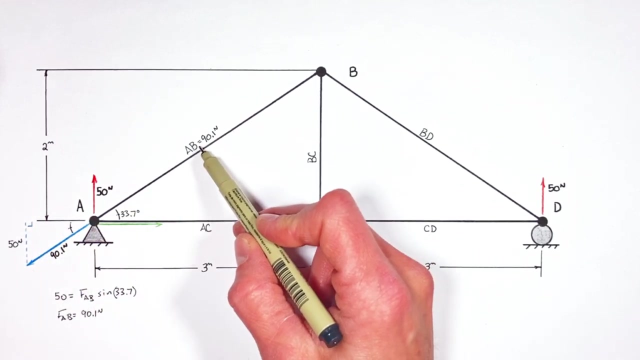 pushing down and to the left on this joint. that means AC has to be pulling to the right on the joint in order to keep the joint from moving horizontally. So solving for the horizontal or right triangle is going to give us not only the horizontal component of AB, it's going to tell us 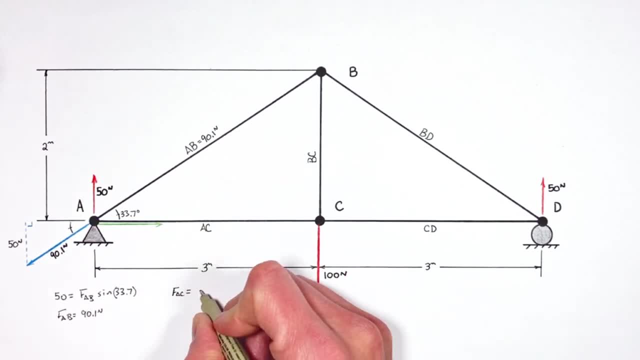 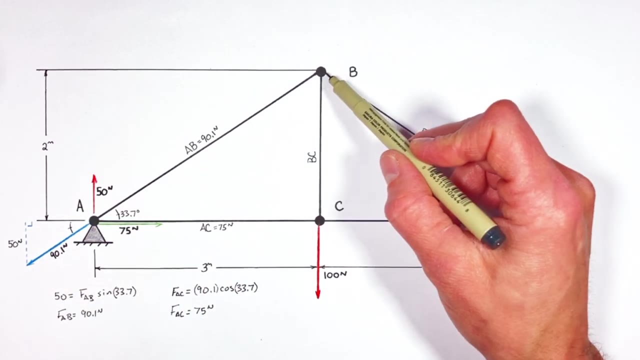 how hard AC is having to pull back to the right. And we find the force in beam AC is 75 newtons. Now the next important rule when solving trusses is that whatever force acts on one end of a beam, like this 90.1 newton, force is also going to act on the other end of the beam. 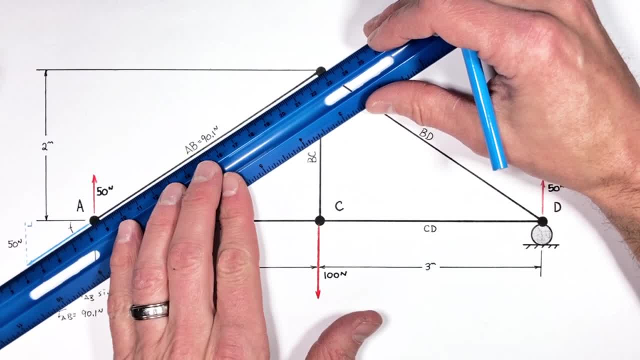 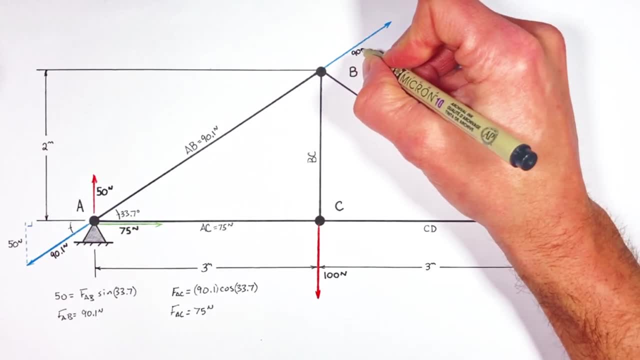 but in the opposite direction. So if there's a force down and to the left on one end of beam AB, there's going to be a force of equal magnitude, but opposite direction on the other end of beam AB. And the same thing is true for beam AC. 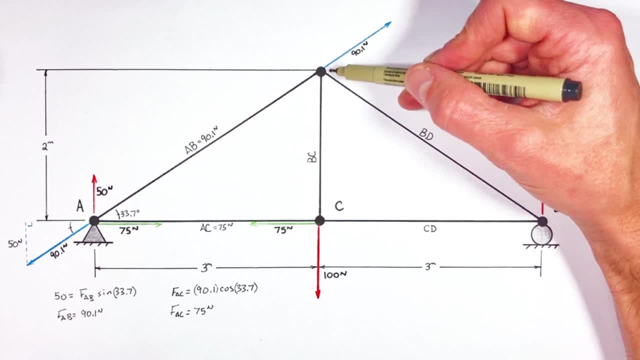 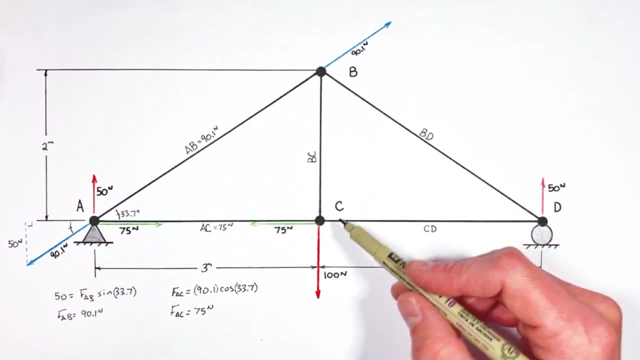 Now it's at this point that we again have a choice. We can either choose to apply the method of joints up here at joint B or down here at joint C. So let's take a look right here at C, because things are already pretty well worked out for us. You see, there's one beam coming in. 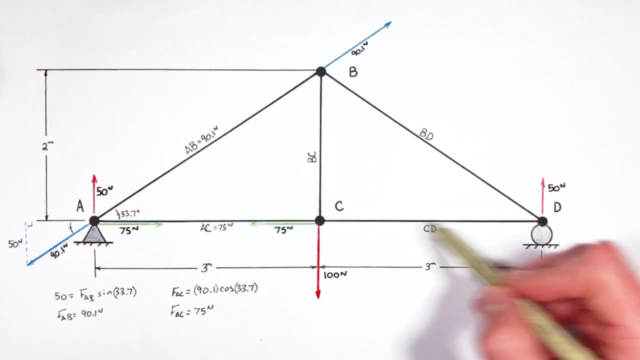 vertically to joint C. here The other two beams are acting horizontally, which means the only beam that's going to be acting horizontally is the one that's going to be acting vertically. beam that can act vertically on this joint right here is BC. So if there's 100 newtons of load, 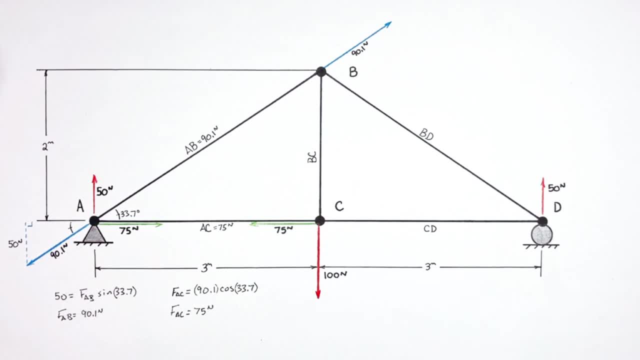 downward on this joint. that means beam BC must be acting upward with a force of 100 newtons. Remember, these other two beams can't act vertically on this joint, They're just horizontal beams. And because beam AC is pulling to the left on this joint C with 75 newtons of force, 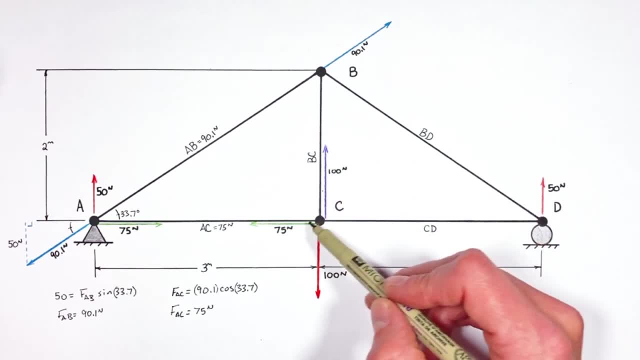 and BC is acting vertically, meaning it can't act horizontally on this joint. that means beam CD must also have a force of 75 newtons in it. So we now know the force in four of the five beams that make up this truss. 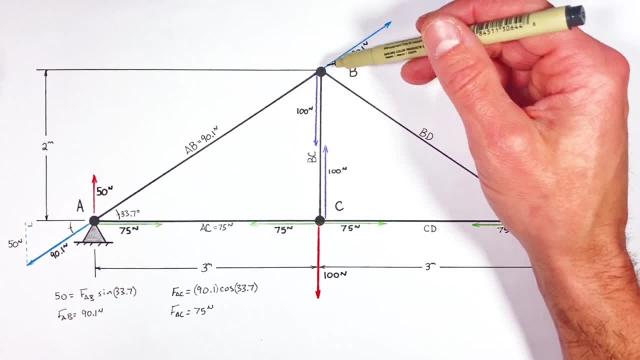 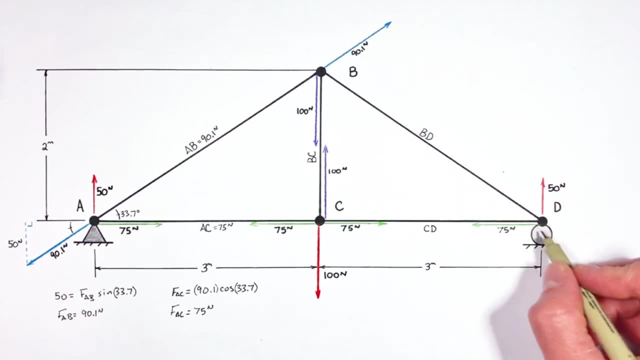 the only unknown being BD. Now, BD acts on two different joints and we can look at either joint in order to solve for the force in BD. So, looking over here at joint D, since beam CD is pulling to the left with a force of 75 newtons, BD acts on two different joints and we can look. 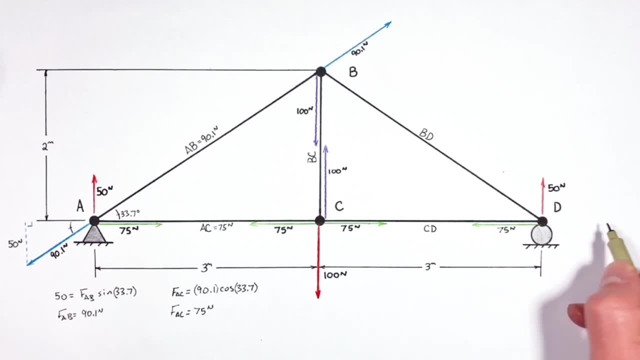 75 newtons, The force by BD must be acting to the right with the same force. And since this support over here is pushing up with a force of 50 newtons, BD must be acting down with 50 newtons of force. So using the Pythagorean theorem we can solve for the force in beam BD And we find: 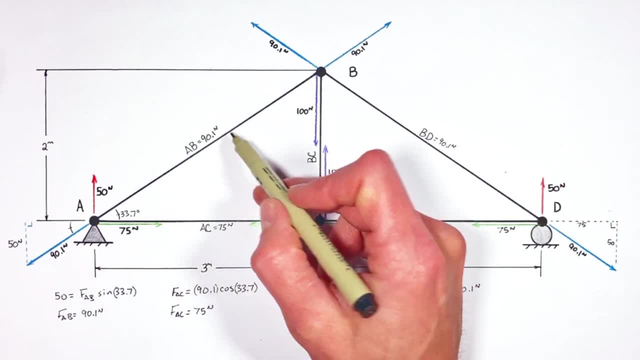 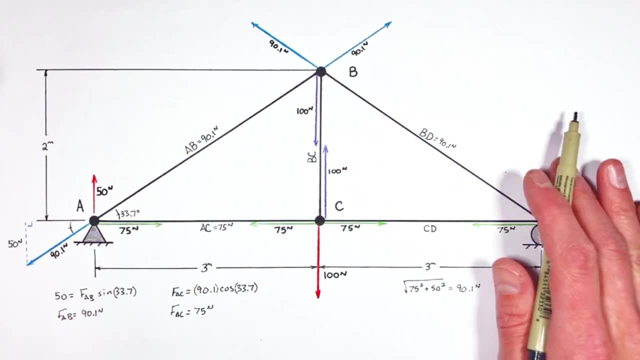 the force in beam BD is the same 90 newtons that were in beam AB, And that shouldn't be a huge surprise, since the force in beam BD is the same 90 newtons that were in beam AB. And that shouldn't be a huge surprise, since the force in beam BD is the same 90 newtons that were in beam AB And that 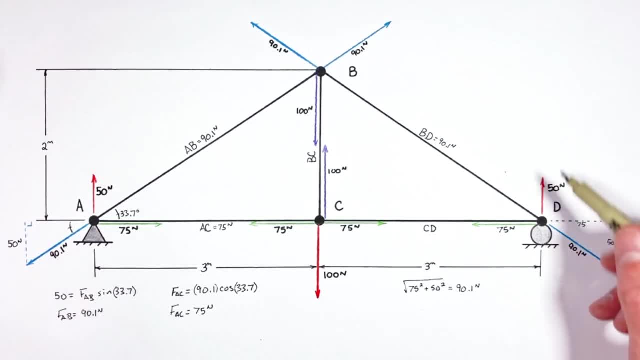 should mirror the forces on the right side of the truss And realize really all we've done. at each joint here is drawn a free body diagram showing all the forces acting on that particular joint. Now to understand tension versus compression, let's take a look at two springs. 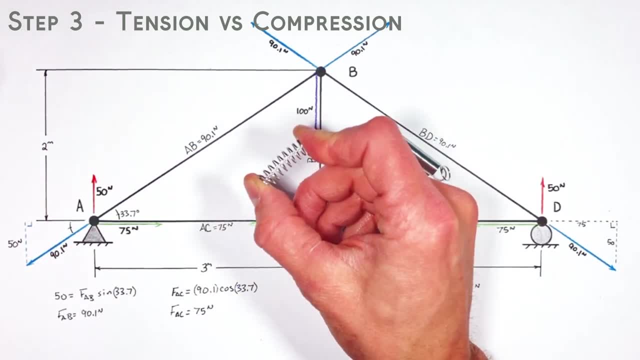 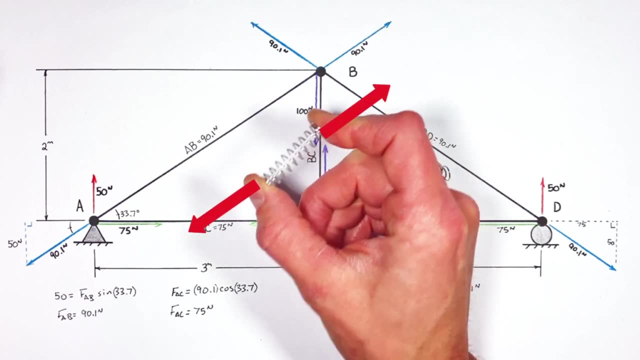 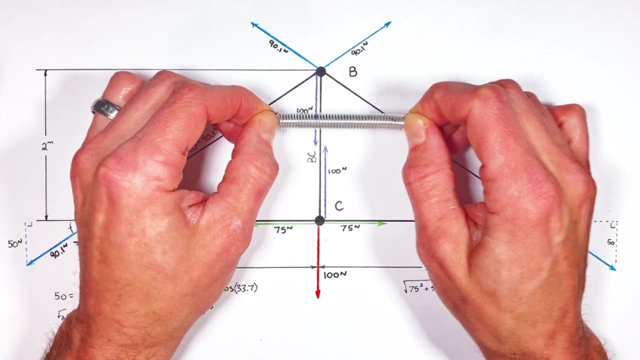 You see this spring right here, we can push on or compress. And when we push on this spring to compress it, this spring itself is pushing outward, trying to go back to its original length. And this other spring we can stretch or put it under tension. And when we